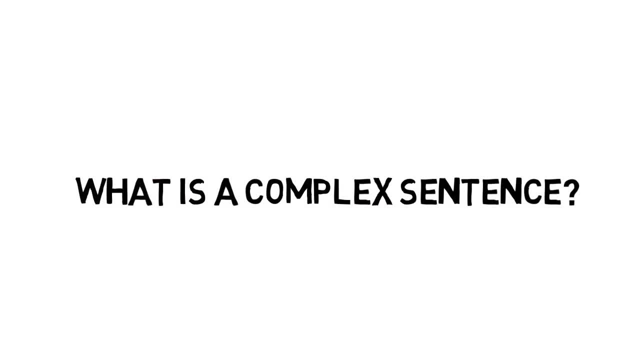 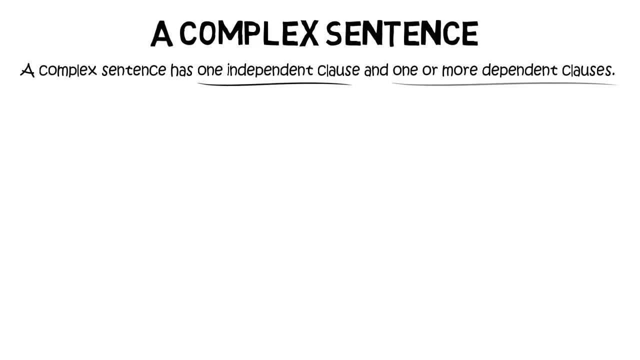 In this video we'll look at what we mean by the term complex sentence. So what is a complex sentence? Well, it's one that has one independent clause or one or more dependent clauses. Now, an independent clause is one that can stand alone as a sentence. a little bit more on that. 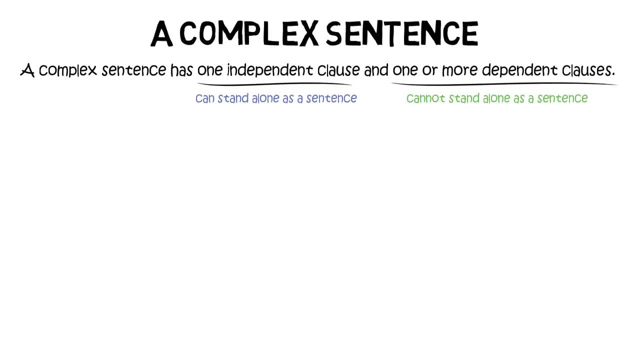 in a second, and a dependent clause is one that can't stand alone as a sentence. So in this video, the independent clauses are all going to be in blue and the dependent clauses are all going to be in green. So let's look at our first example. 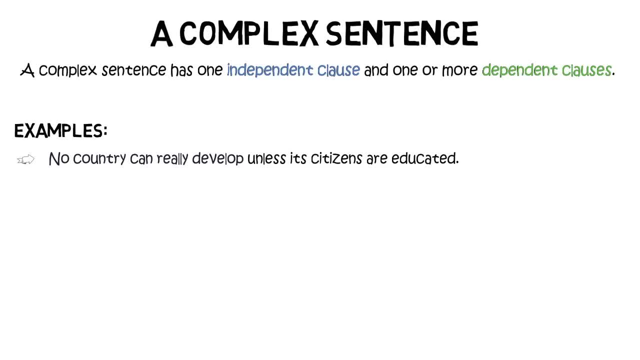 No country can really develop unless its citizens are educated. Quote by Nelson Mandela. So you can see here: no country can really develop. in blue, That could be a standalone sentence. That's an independent clause, And then appended to that in green is the dependent clause, Unless its 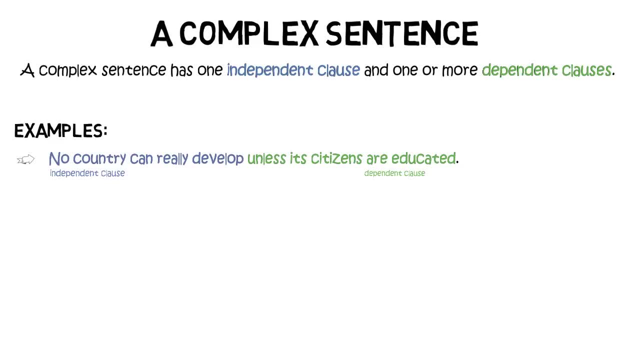 citizens are educated. So unless its citizens are educated is dependent clause, because it can't stand alone as a sentence. Now an independent clause and a dependent clause are joined with a subordinating conjunction and we'll look at those a little later. But in this example 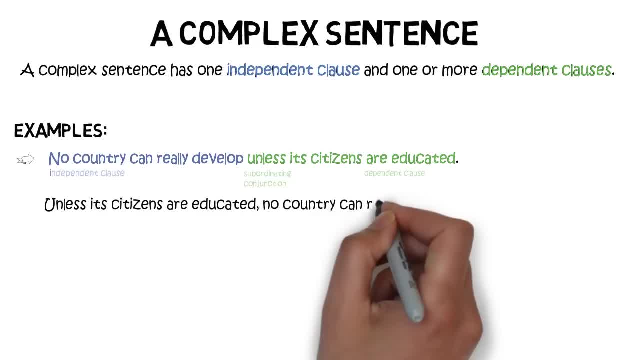 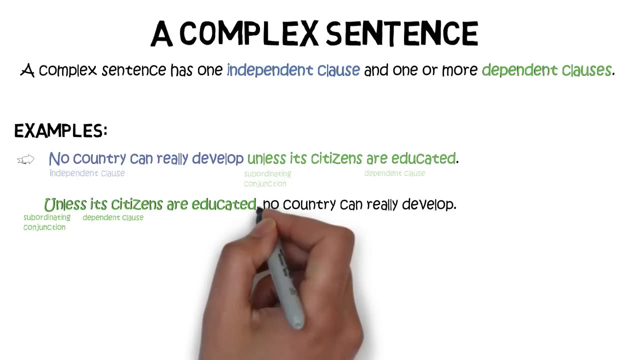 unless is the subordinating conjunction. Now, the dependent clause doesn't always come second. Here's the same example with the dependent clause first. This time it starts with the subordinating conjunction. Unless its citizens are educated, no country can really develop. Let's look at another example. 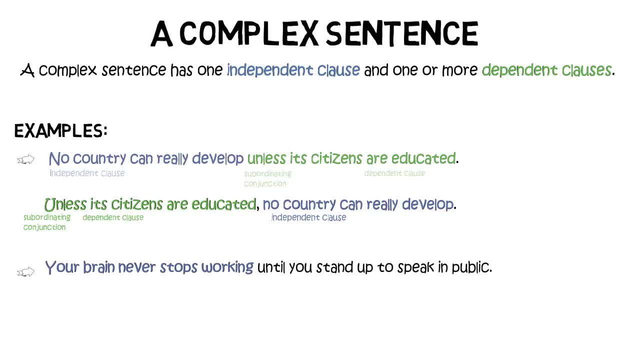 Your brain never stops working. until you stand up to speak in public, Your brain never stops working. That could be a sentence. That's why it's in blue. It's the independent clause And the dependent clause: until you stand up in public. here in green starts with a.